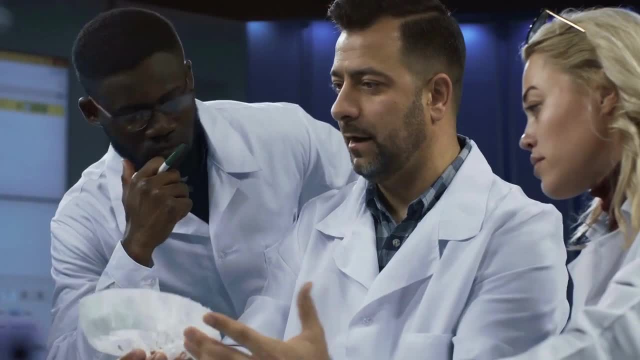 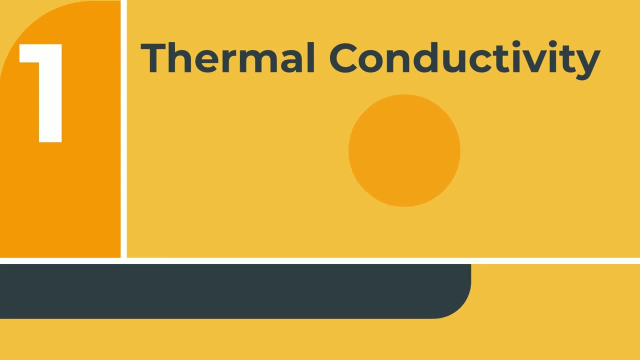 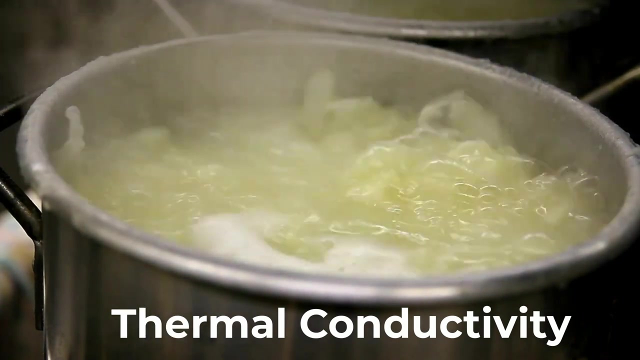 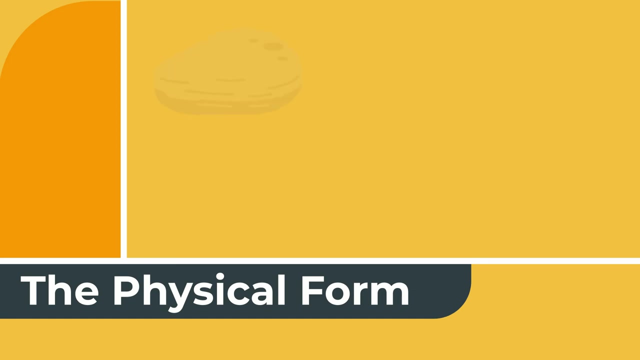 Physical properties are often used to identify objects. Let's take a look at six examples of physical properties. 1. Thermoconductivity: It's the rate at which a substance transfers heat. Metals are very good thermal conductors. 2. State: It's the physical form in which a substance exists, such as solid, liquid or gas. 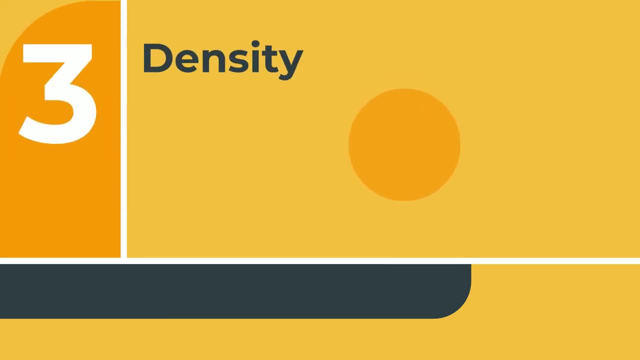 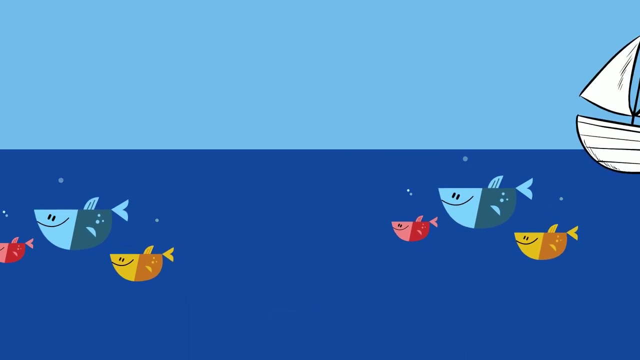 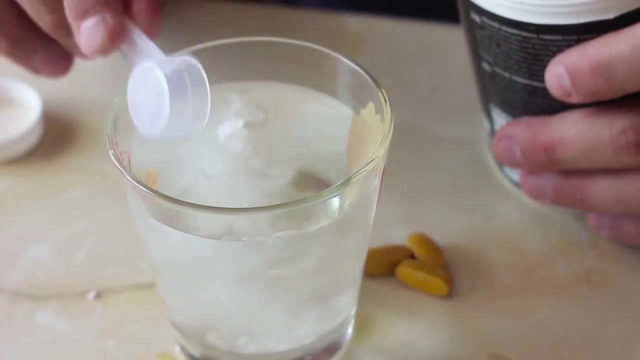 3. Density: It is the mass per unit of volume of a substance. Formula is: density equals mass. Mass divided by volume. An object with a density greater than one sinks and an object with a density less than one floats. 4. Solubility: It's the ability of a substance to dissolve into another substance. 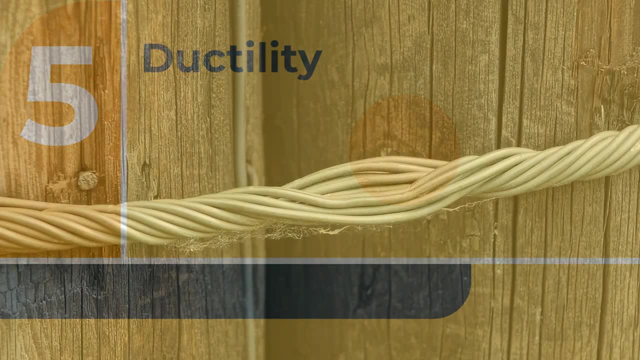 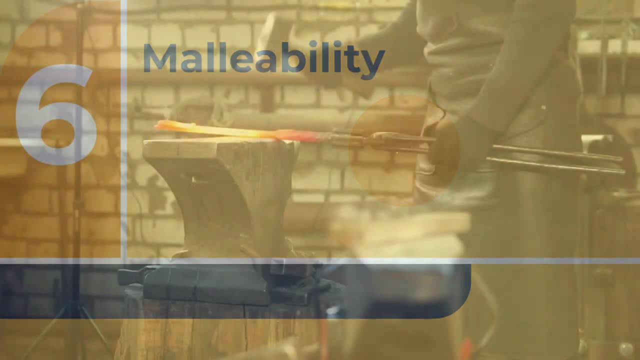 5. Ductility: It's the ability of a substance to be pulled into a wire. 6. Malleability: It's the ability of a substance to be rolled or pulled. 7. Density: It's the ability of a substance to be rolled or pulled. 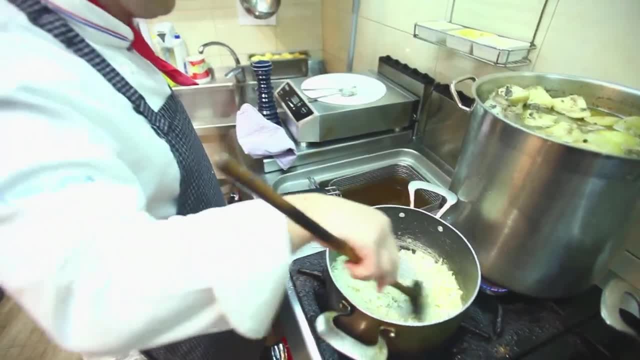 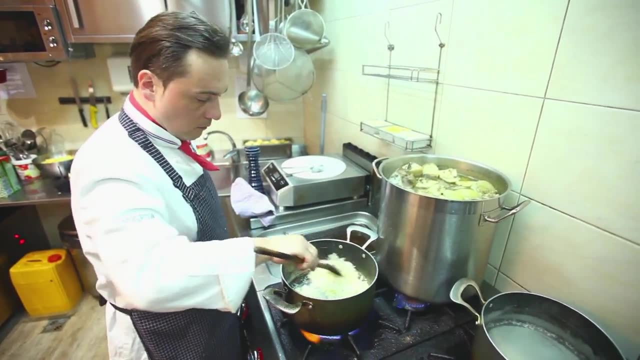 8. Density: It's the ability of a substance to be rolled or pulled. So let's go back to our original question. Why are many pots and pans often made up of metal? Because the metal is a very good thermal conductor and this transfers heat to the food that you are trying to cook. 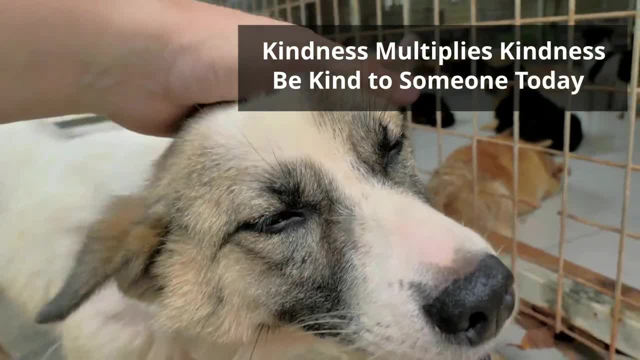 Remember: kindness multiplies kindness. Be kind to someone today.